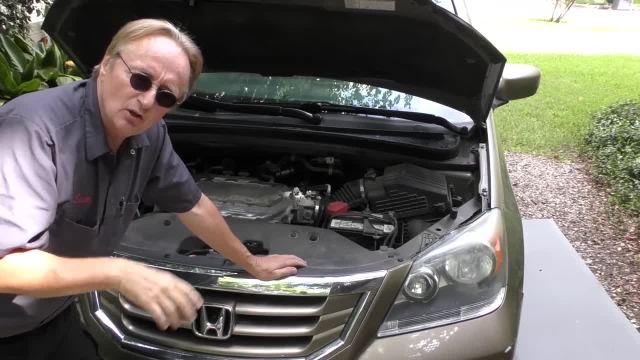 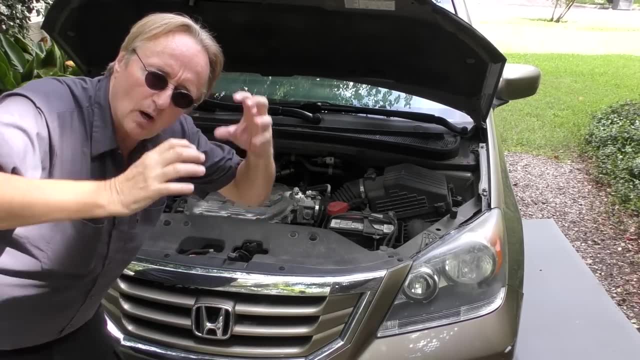 of times the cams wallow out. they start making noise on the backside. there was just something was built wrong in them and the cams that are supposed to spin start wallowing. and then they start wobbling only a tiny amount, but that's. 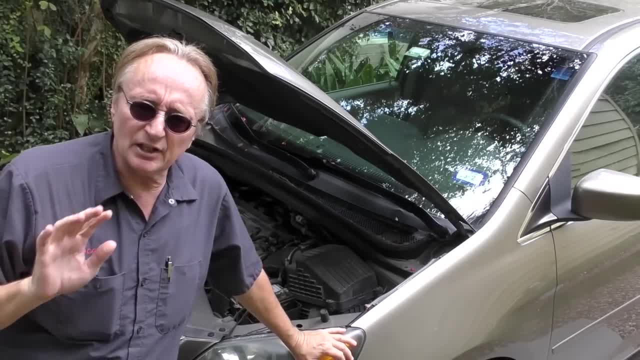 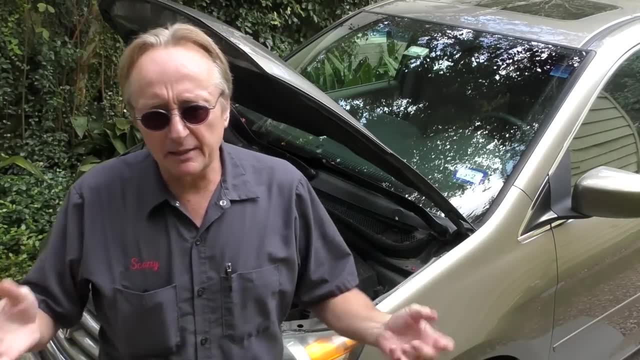 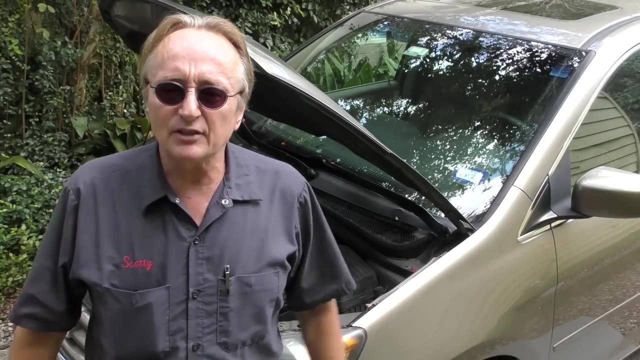 enough to make them make a noise. this particular one. it isn't making the noise very loud yet, but it does burn oil and if you know anything about Hondas, historically they made the strongest engines. I had customers with Civics, Accords, four cylinder engines, 200, 300,000 miles and they would barely burn. 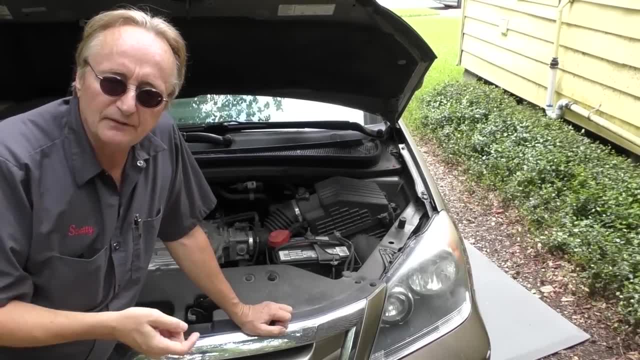 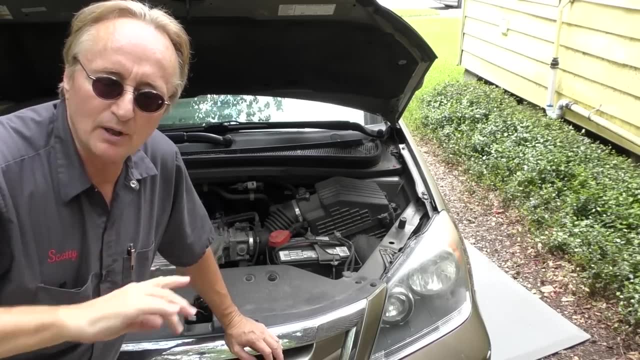 any oil at all between oil changes but this 3.5 liter v6,. if you have engine and transmission problems in the vehicle, that is a gigantic reason not to want to buy one of these, because, after all, Honda Odyssey's main competition is the Toyota Sienna minivan, and those are 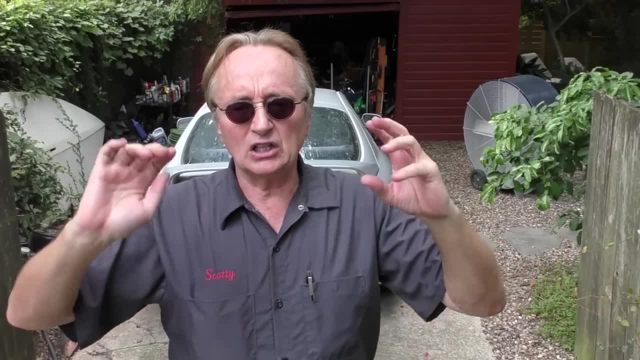 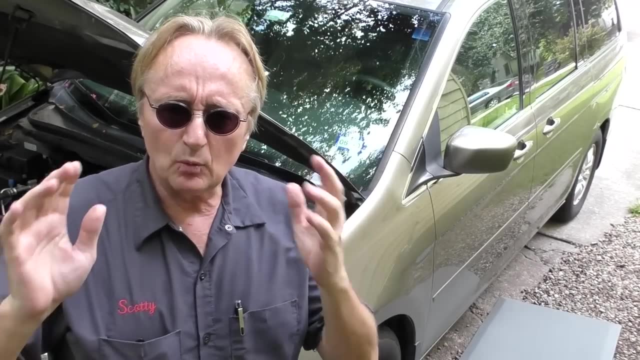 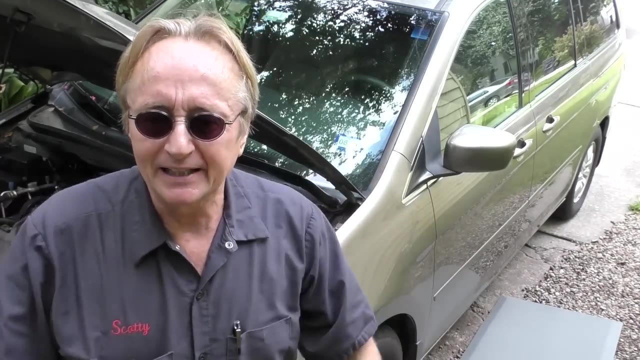 the most bulletproof, long-lasting vans that anybody ever came up with and, hilariously enough, this 2008 van, when it was brand new, it went for $10,000 more than a 2008 Toyota Sienna van. this one was $34,000 and equivalent Sienna was a. 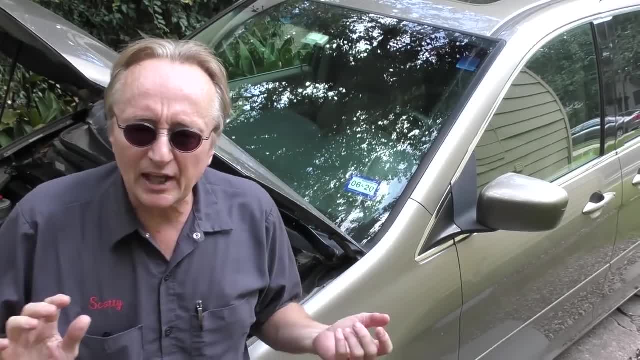 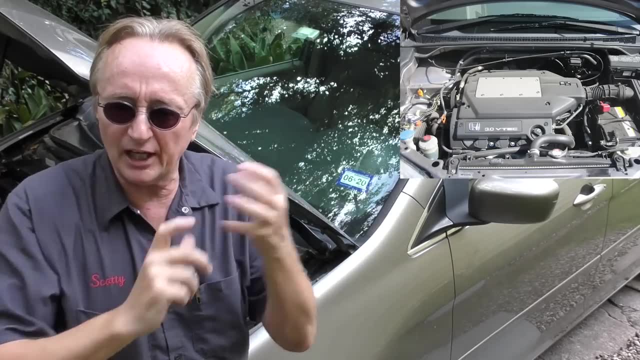 little over $24,000, so in the case of this 2008 Honda Odyssey, you would have paid more and got much, much less: a transmission known for failure, an engine that falls apart, where the Sienna probably would have no serious problems. 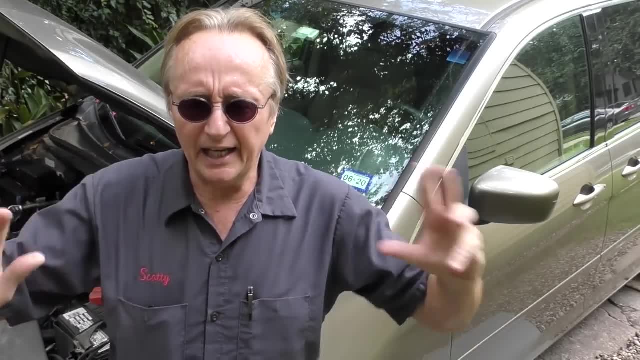 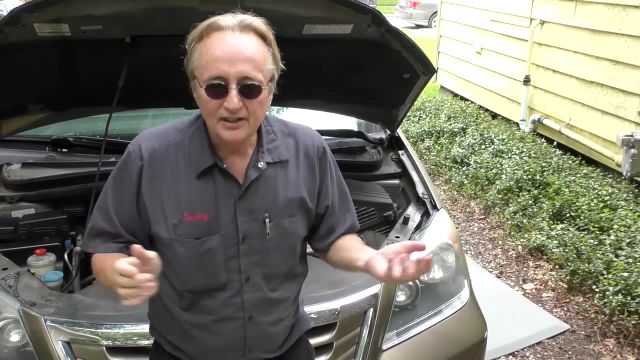 at all these. the trannies go out, the engines go out. what a difference in quality. now, yeah, people like the amenities. it's kind of like the Toyota Sienna, like Chrysler minivans. they sold a lot of them. they were absolute junk. 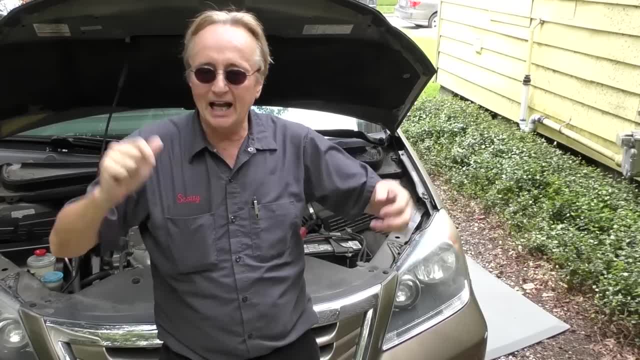 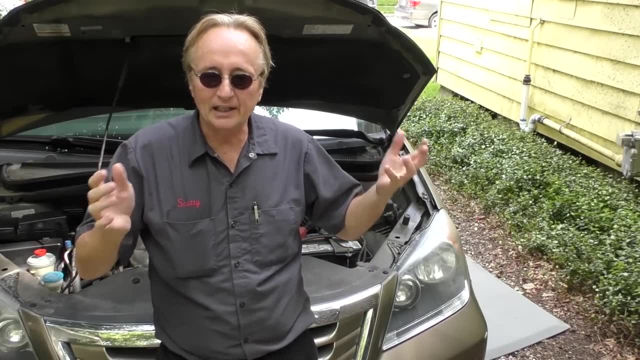 but they had all the cup holders, lots of room, comfy ride video screens for the kids and extra plugs to plug stuff in. they were junk. people bought them because they liked the way they looked and rode, but really they didn't hold up. 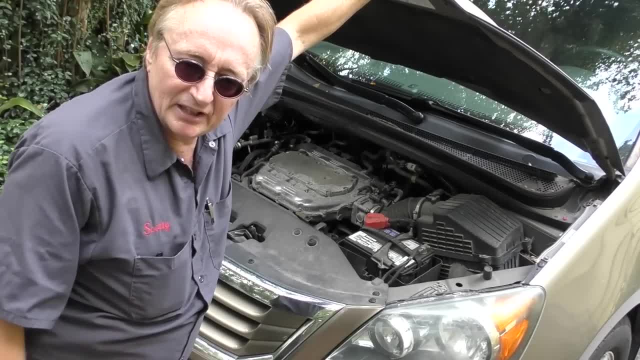 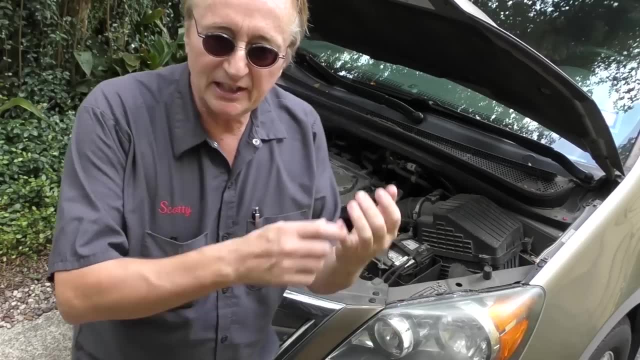 over time. and the funny thing is, these things debuted in 1995 and they were actually better vehicles back then. sure they didn't have all the bells and whistles transmission problems these later ones have. and sure this honda odyssey van puts on a lot more. 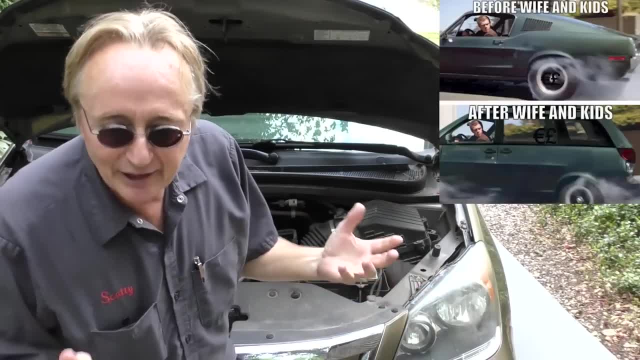 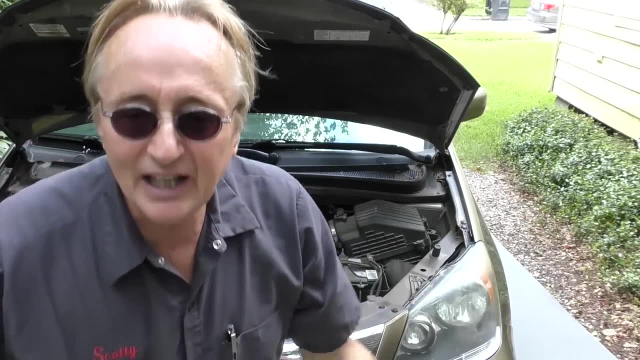 horsepower than a toyota sienna van is. but hey, are you buying a minivan for drag racing or are you buying something for the family that you want to last for decades and hundreds of thousands of miles? minivans are the ultimate practical vehicles. a lot of people laugh. 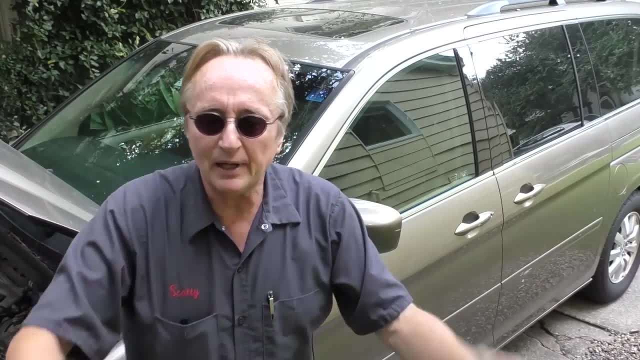 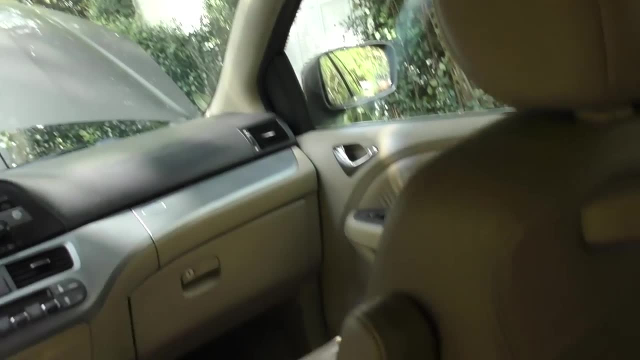 they're just buying a minivan. they live in suburbia. it's a very practical vehicle. why would you buy one that isn't practical because the engine and the transmission goes out and they sure they got a lot of room. this has front seats, back seats, even has third row seats. there's. 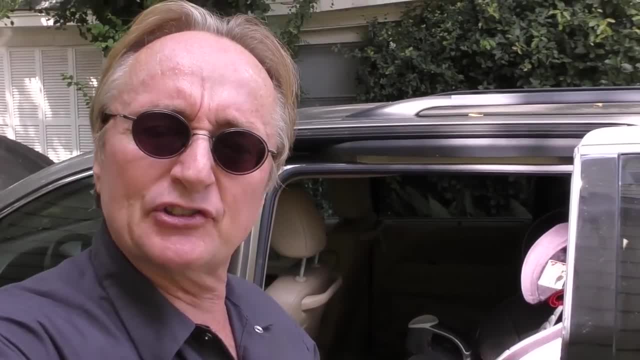 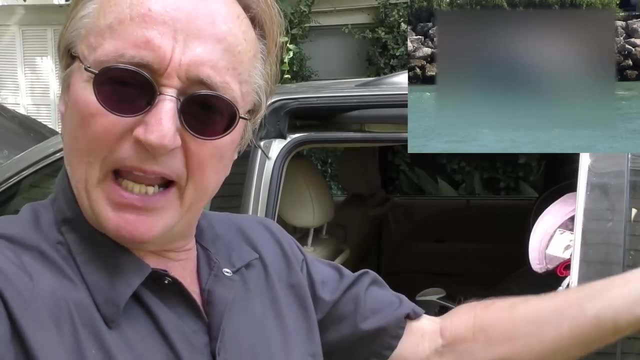 lots of room. there's no arguing that. but if the engines and transmissions aren't dependable, there's no point in buying one, regardless of how comfortable it is, unless you're planning on parking it on the back 40 and living in the thing and not actually driving it around. 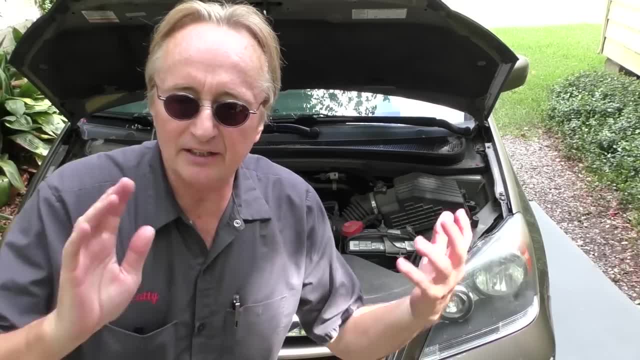 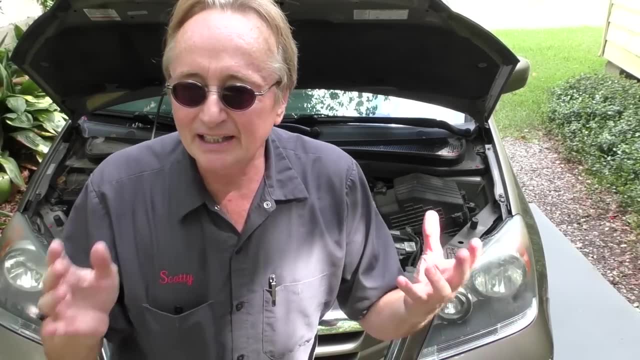 and yes, these odyssey vans, they handle better than the sienna vans. but you want practical quality. you don't want something that you're taking on a race car, you want something that's going to get you from here to there. now, sure, they're nothing as horrid as the chrysler minivans. 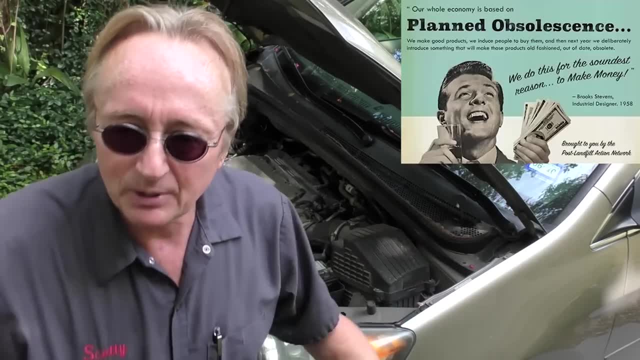 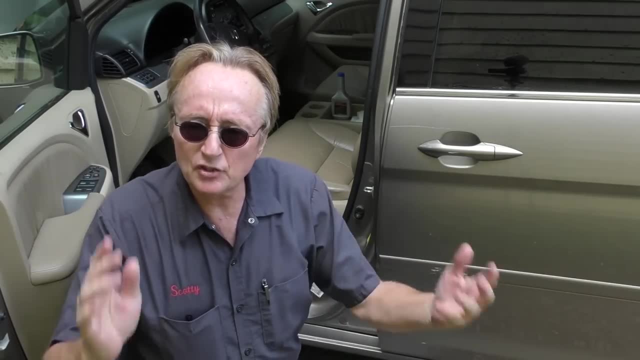 i mean, those are just instant self-destructing vehicles, planned obsolescence taken to the nth degree. and most people are buying a honda. they're assuming they're getting a japanese product made in japan, but not in this case. we'll go down the door to the sticker and what does it say? 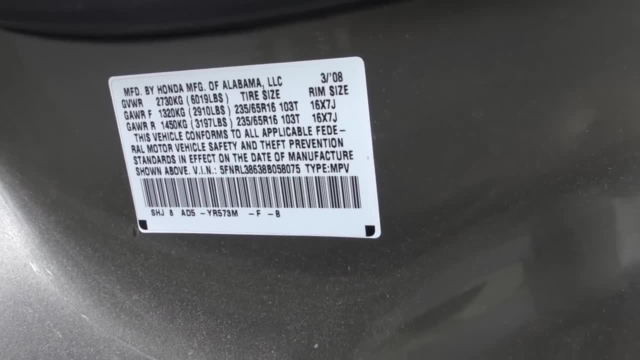 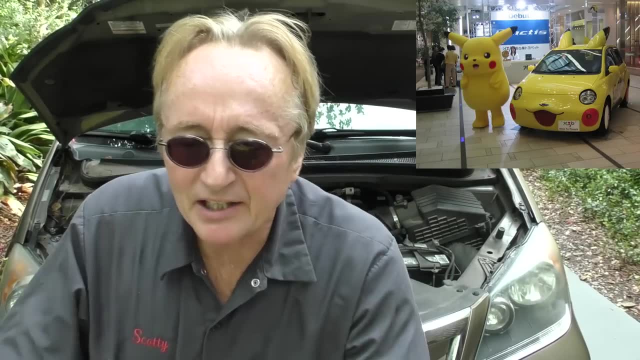 manufactured by honda of alabama llc. it is not made in japan, it's made in alabama and, as i've always said, if i want a japanese car, i want one made in japan by the japanese. just like if i want an italian pizza, i want a pizza. 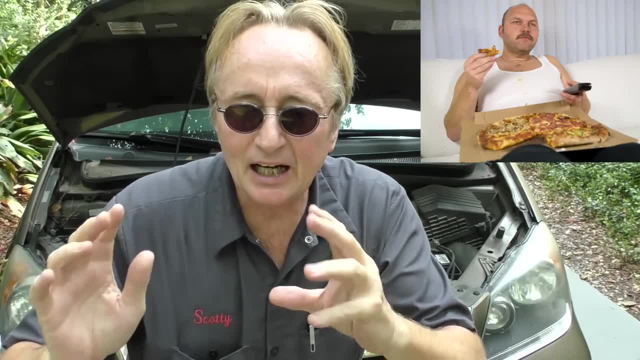 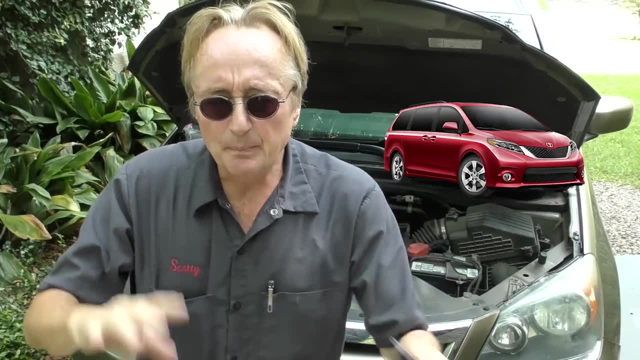 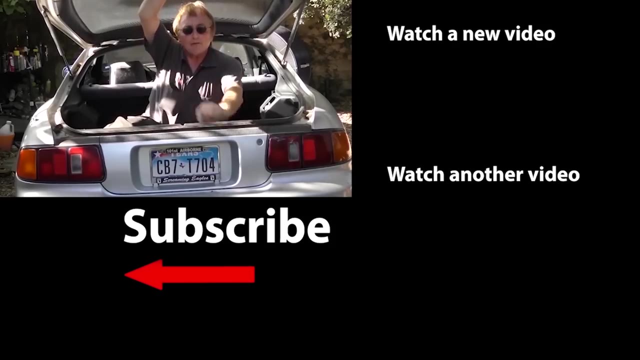 made by an italian, or at least an italian american from new york city. so now you know the reasons why i would not buy a honda odyssey van. there are just better ones out in the market for less money that'll last longer. so if you never want to miss another, 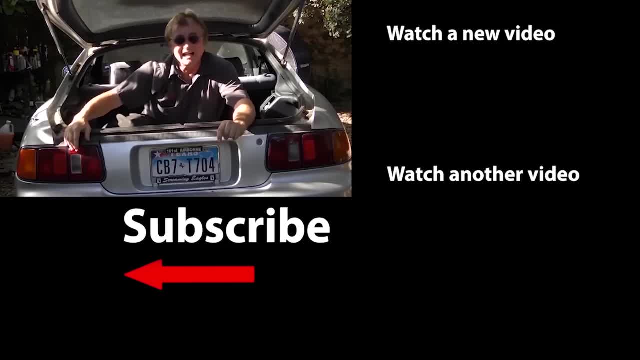 one of my new car repair videos. remember to ring that bell.